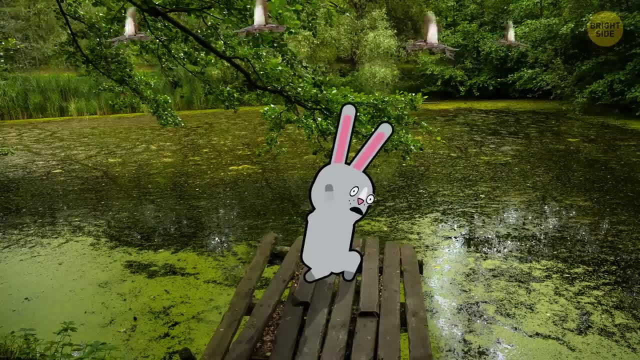 can fall to the ground. They can fall to the ground. They can fall to the ground. They can fly. So don't just watch out below, because they can come from the sky. As you catch your breath on the shore, something lands on your shoulder. 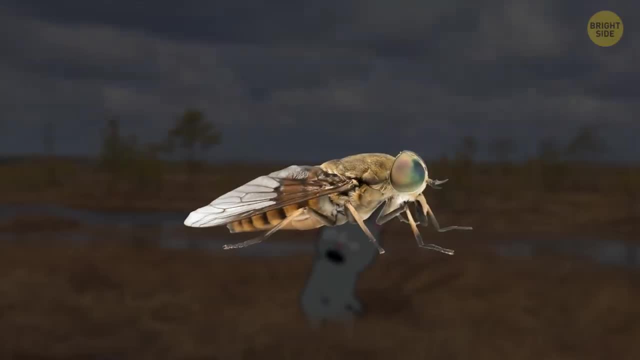 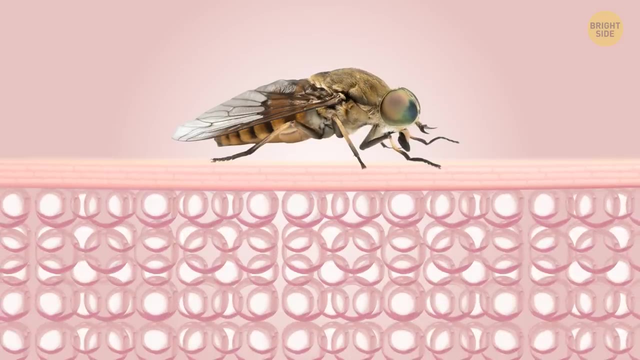 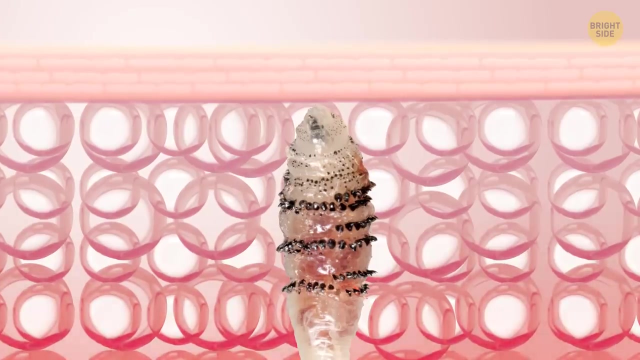 Quick swat it away. It's a botfly. Botflies are vicious tiny insects that lay their eggs and mosquitoes injecting those eggs into humans. Your warm body temperature creates the perfect incubation environment. When they hatch, they start their lives with the grueling task of eating their 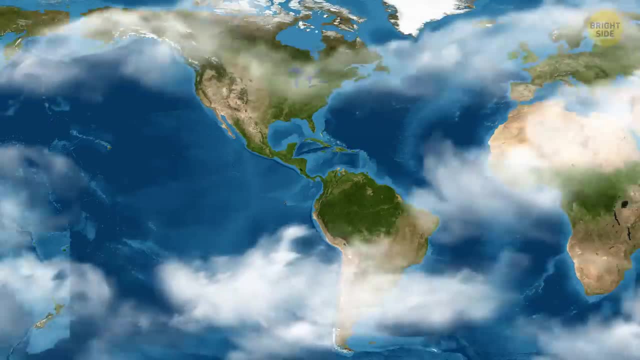 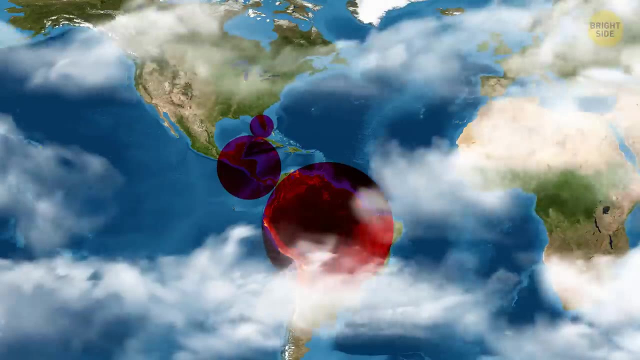 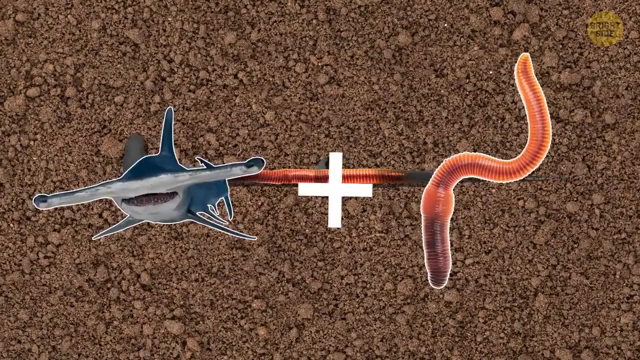 way out Lovely. You're most likely to find them in Central and South America, but it's not implausible for you to have an unlikely encounter with these small creatures in Florida as well. The name hammerhead worm calls to mind nothing good. It sounds like an impossible cross between. 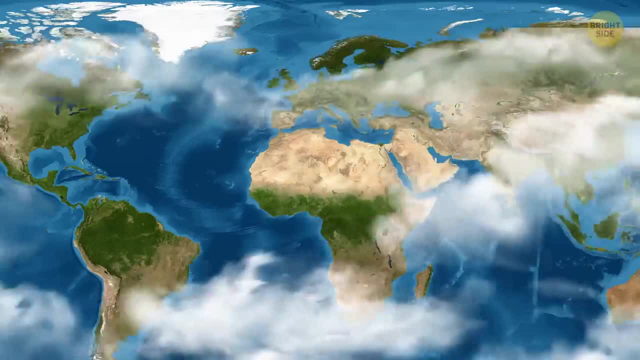 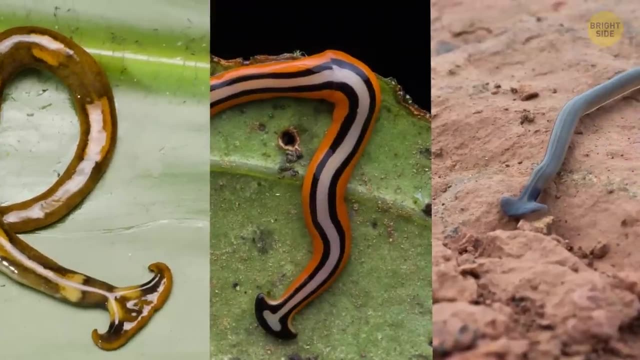 a shark and an earthworm Looking at one that's not far off. Multiple sightings of this strange creature were reported across Georgia. They live up to their name With a distinct crescent-moon-shaped head. well, what appears to be their head? 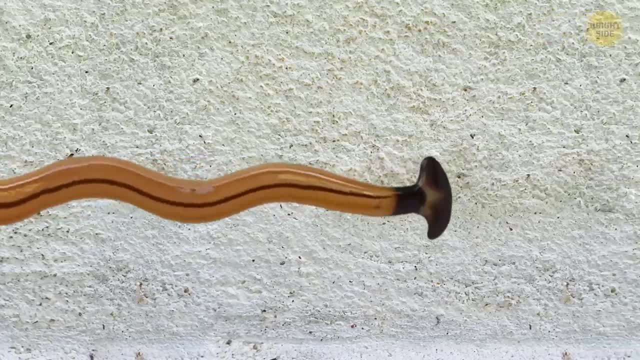 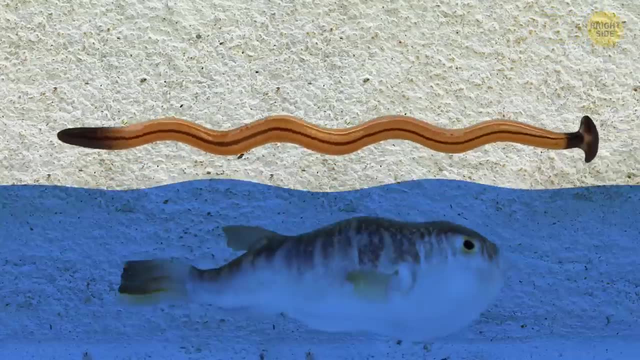 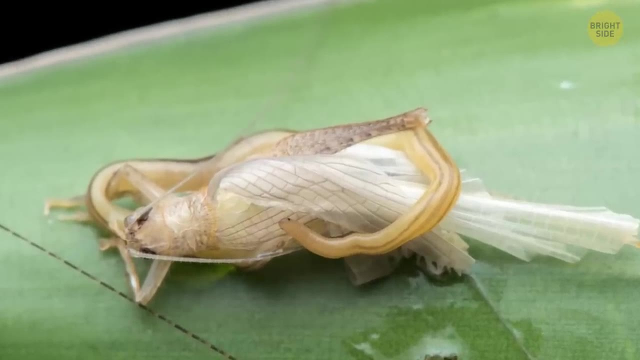 their mouth is halfway down their bodies. Their appearance is off-putting for a reason. These babies are poisonous. They produce tetrodotoxin, the same as pufferfish. Scientists aren't yet sure how it uses the toxin, but the best bet is that it's a tool to catch its. 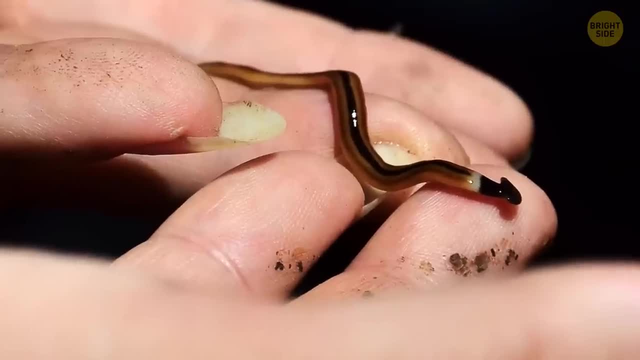 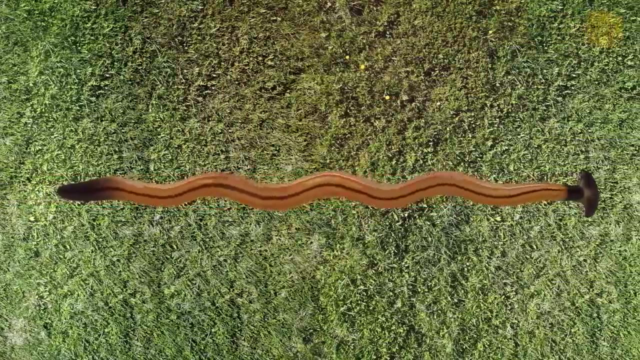 prey other worms. We also don't know how much of it would hurt a human, but experts say to stay away no matter what. If you want to know more about these creatures, click the link in the description. Especially, don't harm it, because it has the spectacular ability to reform itself. 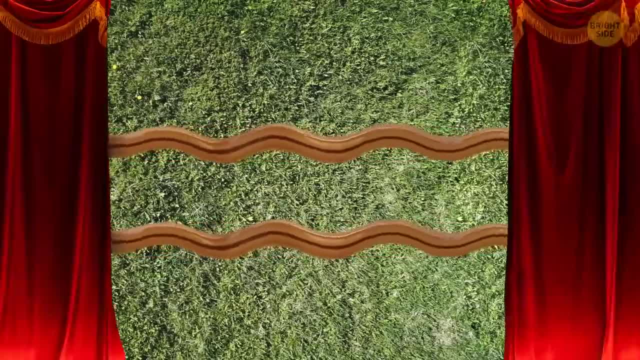 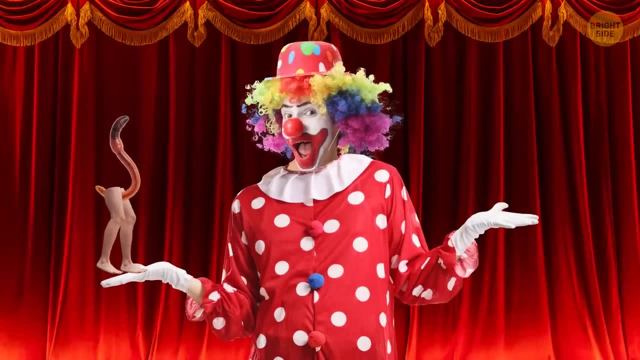 out of cut sections of its body, like the myth of the hydra. Side note, someone with a great sense of humor nicknamed these grubs lanchovies, which sound much less scary than hammerhead worm, The giant silkworm caterpillar. 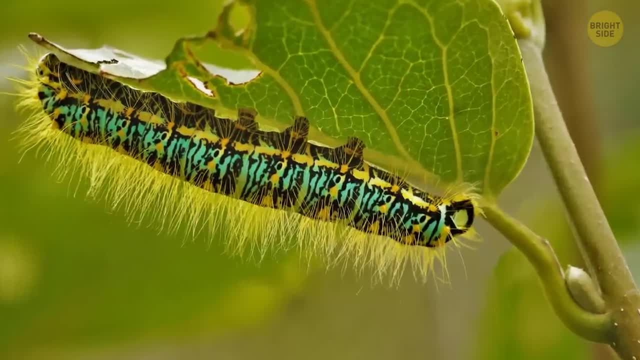 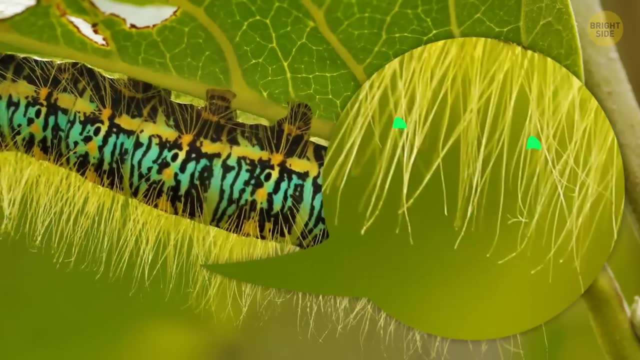 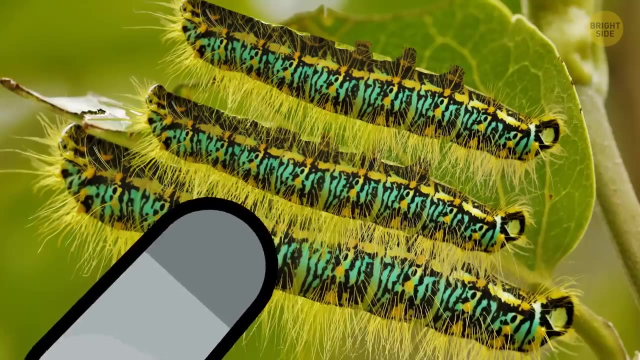 looks as intimidating as it should. Its potent venom is no joke. The larvae are sheathed in tiny vessels which release a highly poisonous anticoagulant toxin. So getting pricked by one of these isn't ideal. but they make it even worse by gathering in bunches, so it's common to 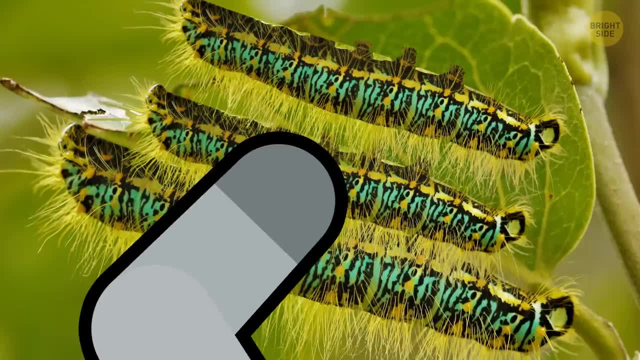 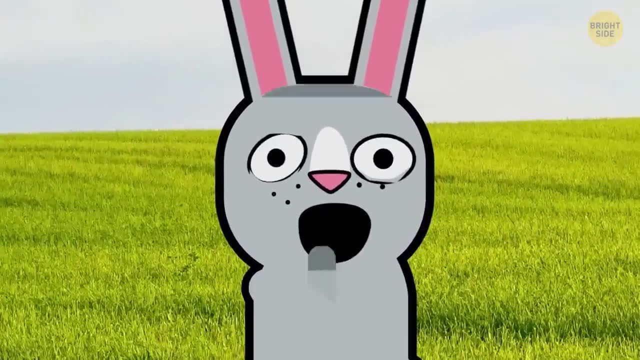 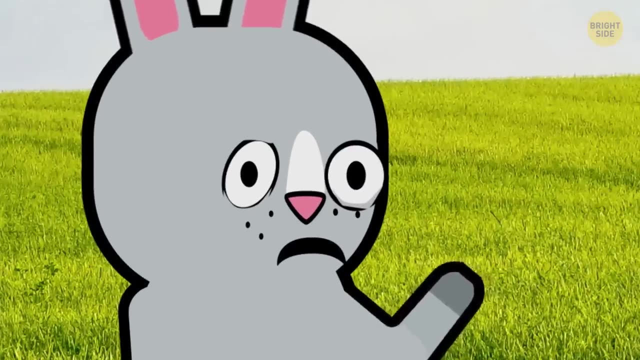 accidentally brush up against multiple caterpillars at the same time. Most people who are stung don't feel it. That's good, right? Well, no, It means they have no idea what's going on when symptoms appear. Plus, there's no visible mark left where they've been stung. 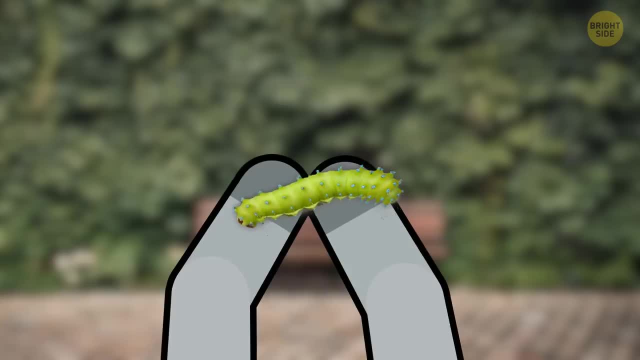 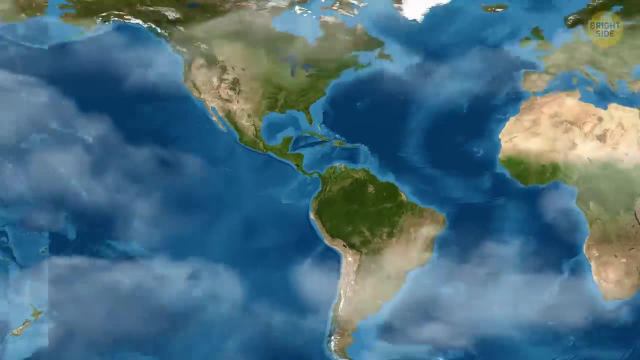 One of the strangest things about this caterpillar is that it's super tiny compared to the damage it can cause, usually around two inches. They're commonly found in the rainforests of South America, including in Uruguay, Argentina and Brazil. But plot twist. 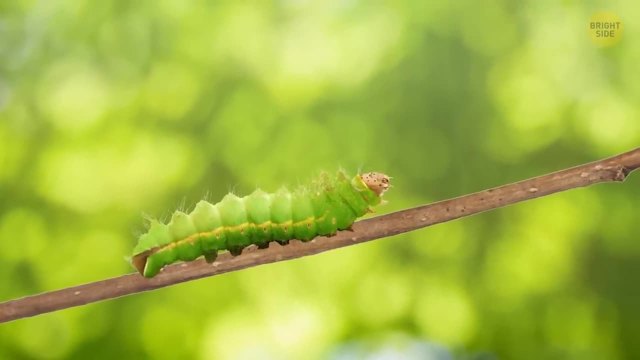 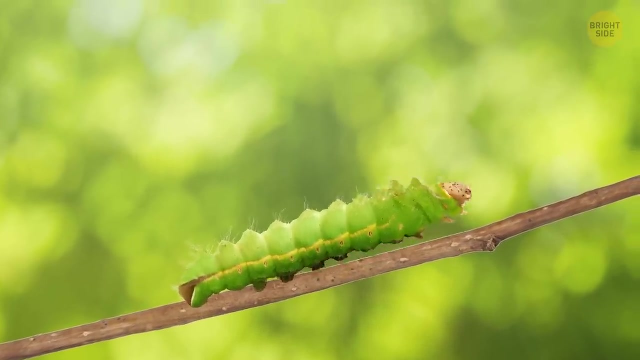 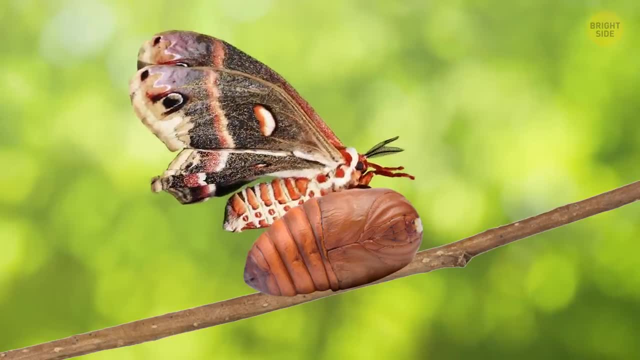 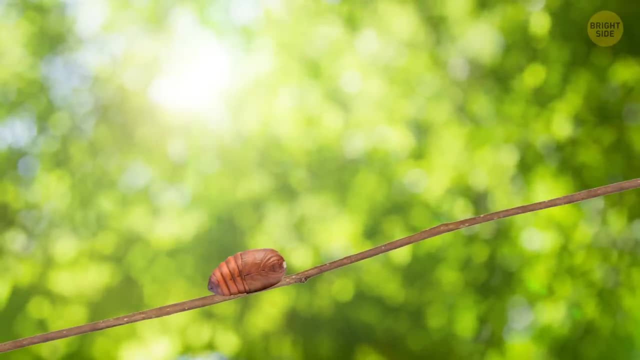 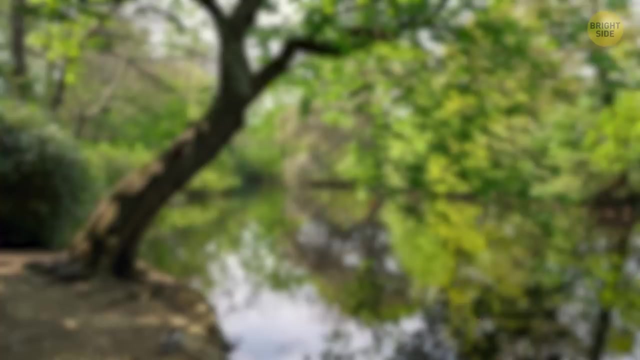 silkworm moth. But don't be fooled into thinking it's harmless now because it's lost its vicious spikes. It's still venomous and now it can fly. You can take comfort in knowing that it only lives for a few weeks in this form, though, because once it metamorphoses, it no longer has a mouth. 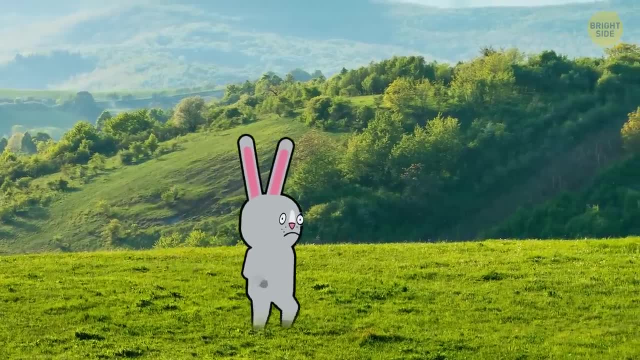 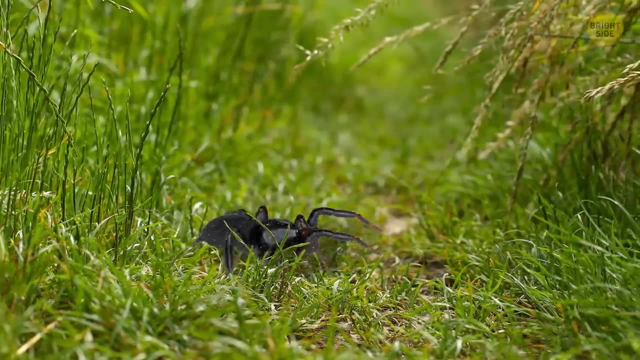 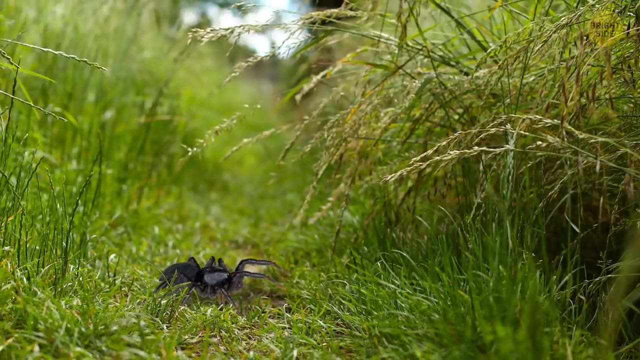 to eat with. The Australian funnel web spider toxin can take out an adult human in about 15 minutes. That's why it's widely considered the world's most dangerous spider. While all funnel web spiders are no darlings, this specific species takes the cake They're. 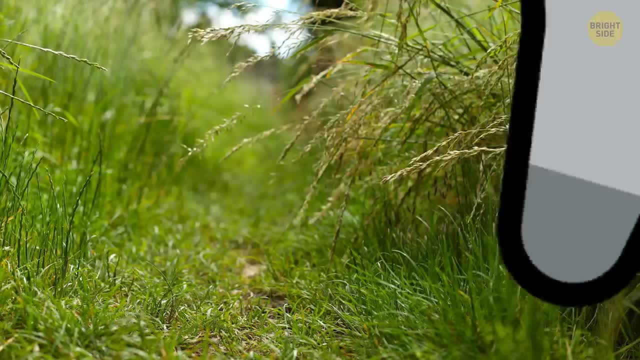 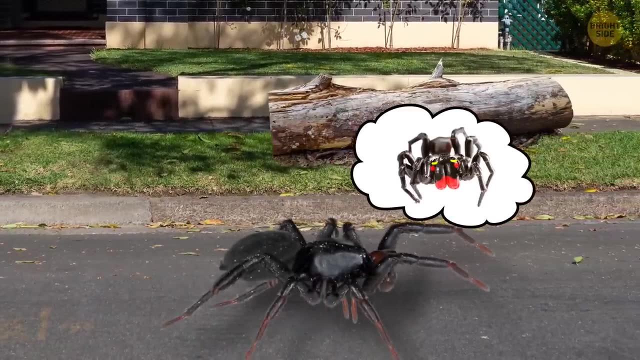 relatively large and aggressive, with rear-facing fangs capable of piercing through your fingernails. The males often wander into human-populated areas in search of mates and are much more likely to cause harm. They make their burrows in cool, sheltered areas. 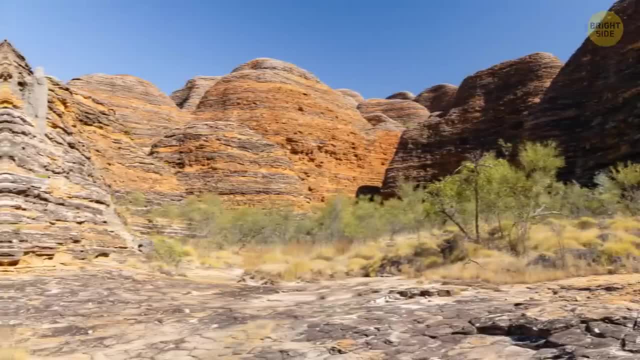 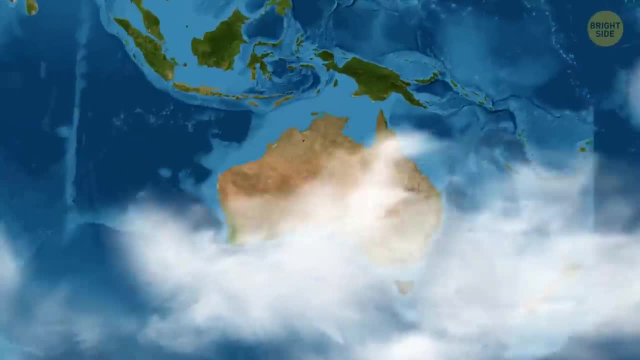 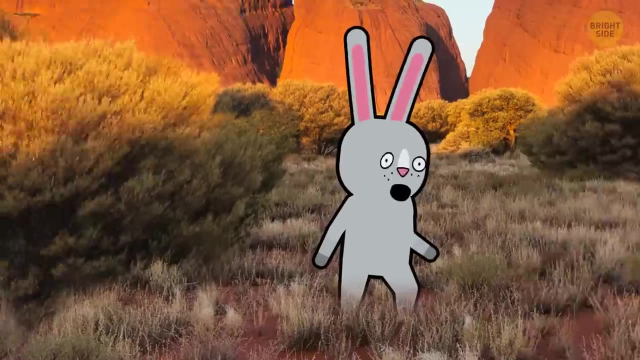 such as under rocks and inside rotting logs. Worst of all, they're commonly found in shrubs and rock groups in suburban districts. If you're not from Australia, you can feel relief, since they're exclusively native there. If you are from Australia, pay close attention to your surroundings. 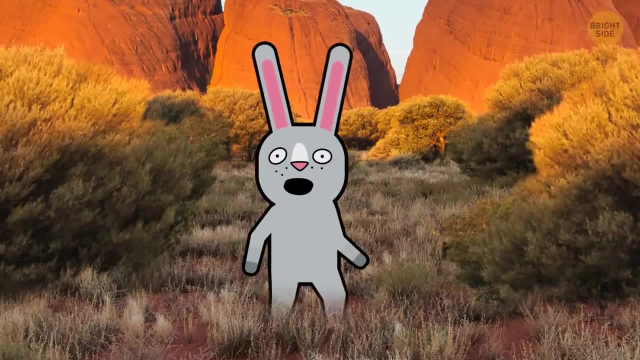 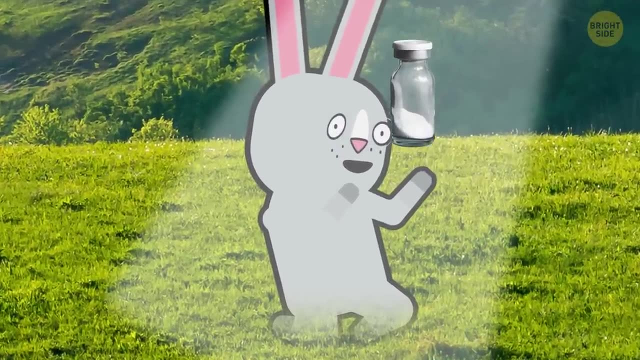 and if you see one of these, stay far, far away. A word of good news: an antivenom was developed in 1981.. Still, it's best to steer clear Down on the bottom of the ocean in tropical areas. 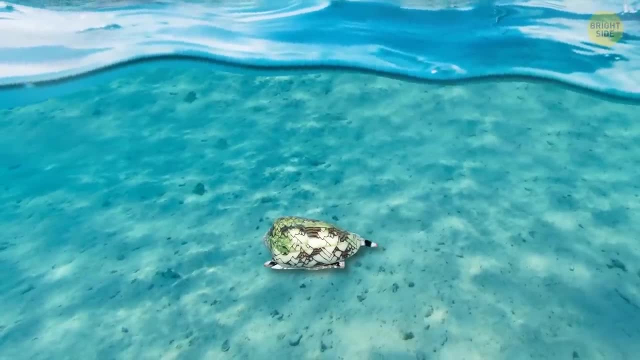 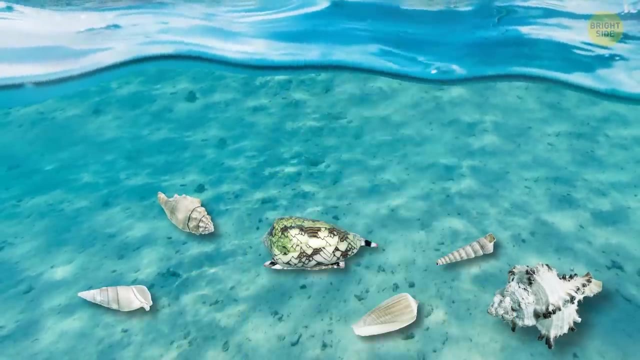 you might spot a beautifully patterned shell like this one. They come in all colors and sizes and look like tiny pottery vases made by little underwater potters. If you're like me, your instinct might be to reach out and pick it up. 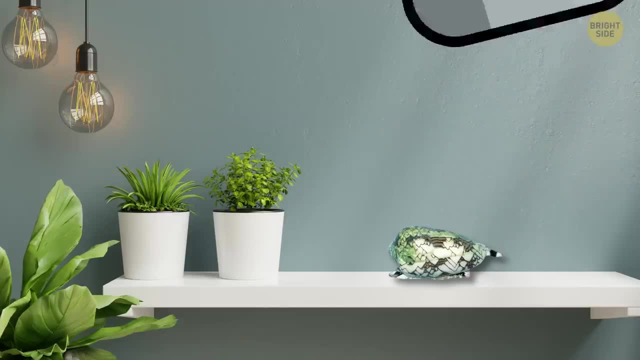 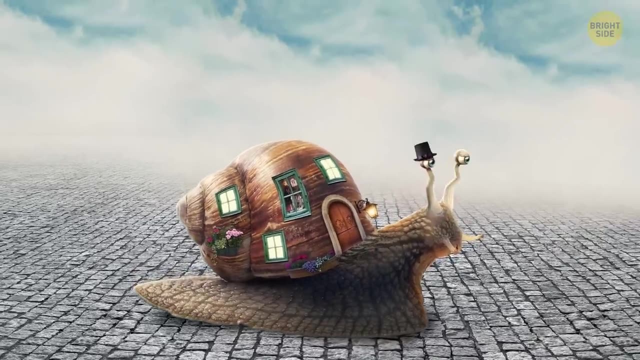 and take it home as a souvenir. That's the last thing you ever want to do. This isn't just any old shell. It's the home of a cone snail. If that name doesn't strike fear into your heart yet, it will soon. Like most snails, the cone snail is slow, but it makes up for it with calculated moments of dangerous swiftness. They're predatory, seeking out other snails, fish and marine worms. They sense potential food nearby using their nose and deploy a sharp, needle-like proboscis. 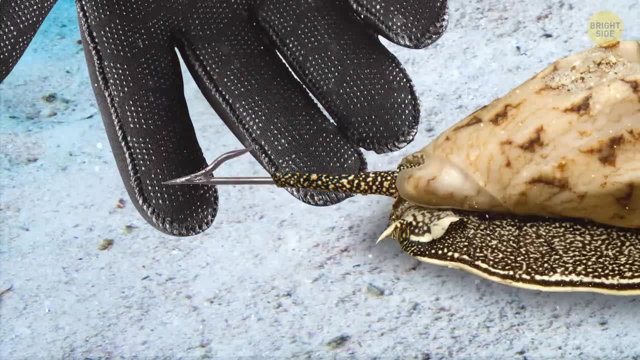 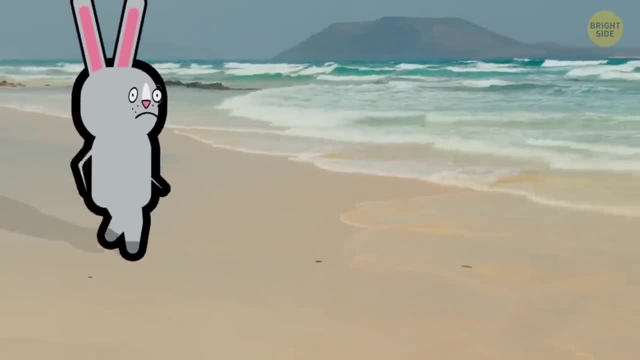 to spear their prey. The harpoon-like beak is strong enough to penetrate fabric, even reinforced diving gloves. If you're a human- and I sure hope you are- you're not the cone snail's ideal meal. That doesn't stop it from stinging people that get too close If it does. 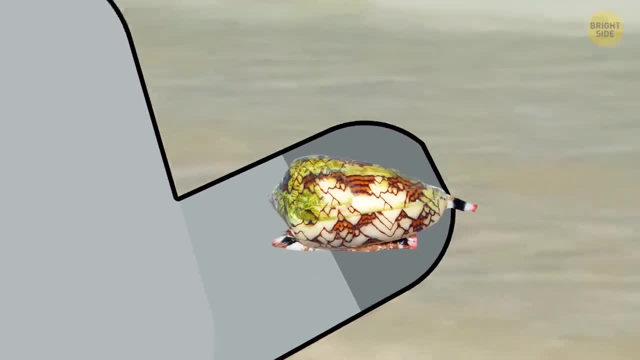 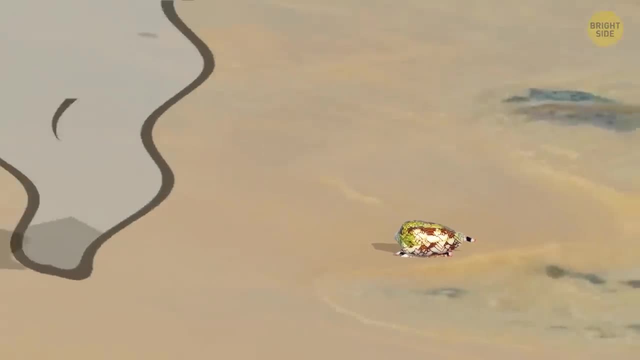 sting you, you probably won't feel it because the venom that is injected in that instant is laced with a natural pain reliever. The lack of pain is actually what makes this snail so dangerous. Without knowing what's hit you, you may not register the sting symptoms until it's too late. 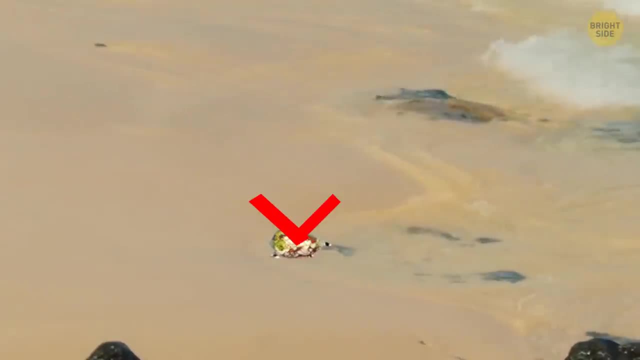 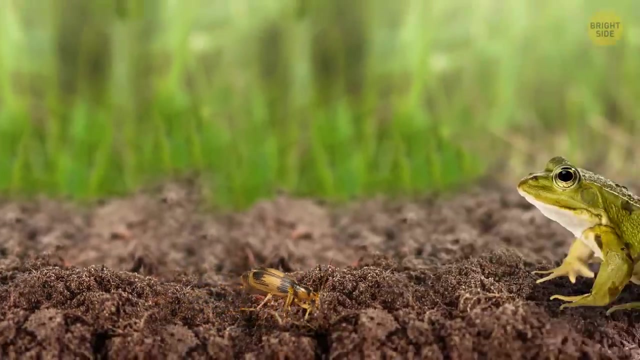 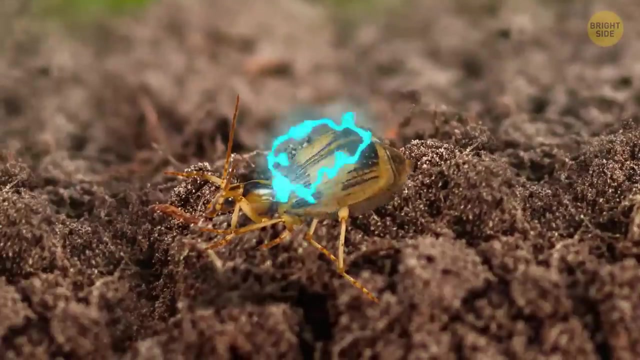 So if you see a pretty shell, stay safe by leaving it be. This miniscule bombardier beetle has a unique talent: When threatened, it can shoot boiling hot, poisonous acid from its backside. It uses the stinky chemical spray to ward off predators and lash out against other insects. 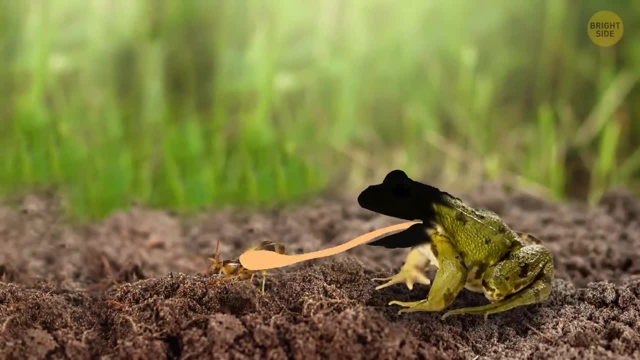 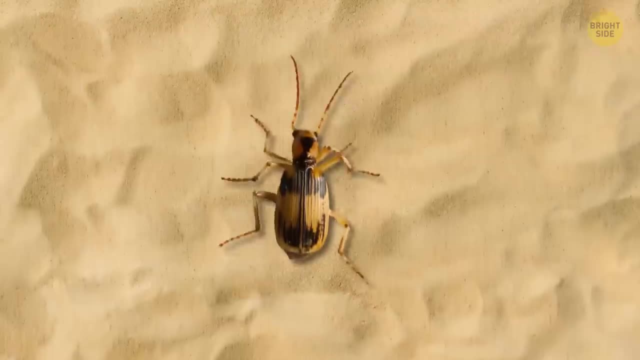 And it works well. Sometimes it even saves their lives. after they've been swallowed, Frogs will often spit them back up once they taste their less-than-pleasant flavor. You might find one in many different ecosystems, from deserts to grasslands to thick forests. 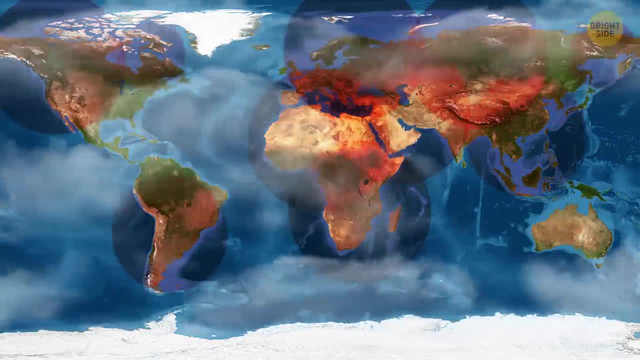 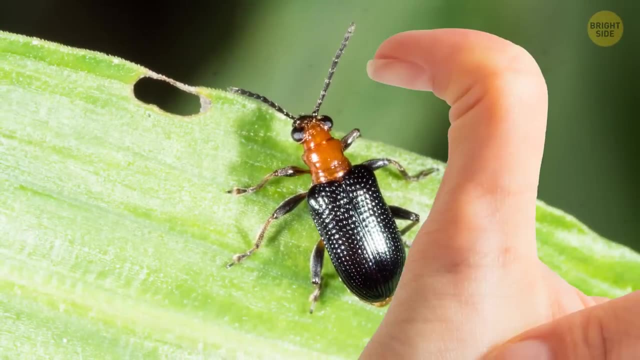 They're so versatile that they're found on every continent except Antarctica. You've probably never noticed one before because they're so tiny, only about the size of a fingernail. Incredibly a potent spray can come from such a little bug.